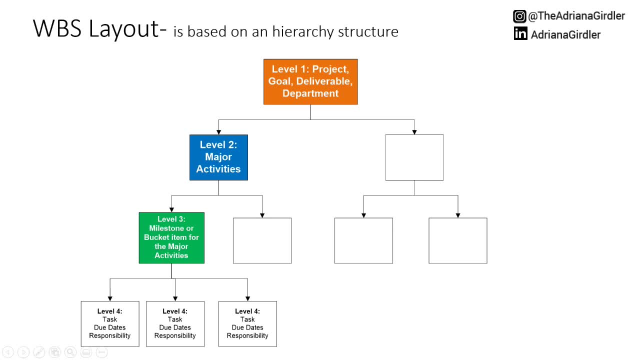 an org chart. So, like an org chart, your top level would be your CEO or your president, as we have here. But for the WBS it's actually the project goal. It could be a deliverable, a department. You can break it up whatever you want, but it's really ultimately, if you were to complete. 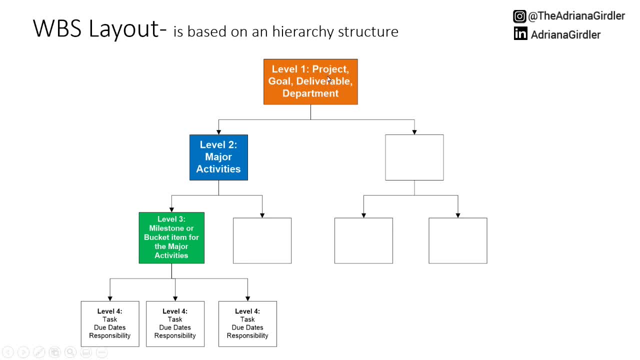 everything. what is it that you're delivering And that's what would be in that particular area. Now you would break it down just like an org chart: You have your president and then you have your VPs or your directors, And it's the same thing here. Your level two would be major activities. 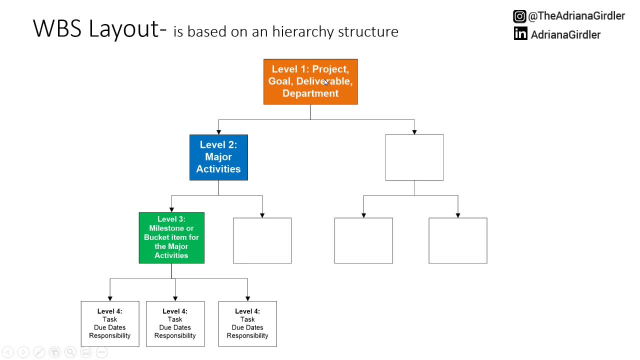 So, whatever that deliverable may be, or department activity, you would break out the major activities- I like to call them the really large buckets, And then you go down to level three. So these are either milestone activities within that major one, They could be even a further breakdown of 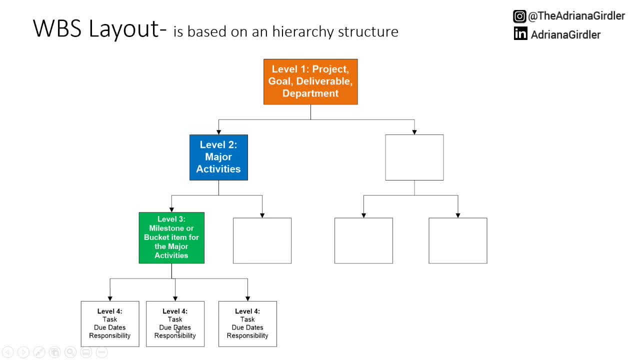 the project. And, last but not least, you have your level four, Those individuals. if you really were to compare it to an org chart, it would be those who were the doers. It's the tasks, It's the orientation. So that's what your level four would be. So, when you have a project, really break it. 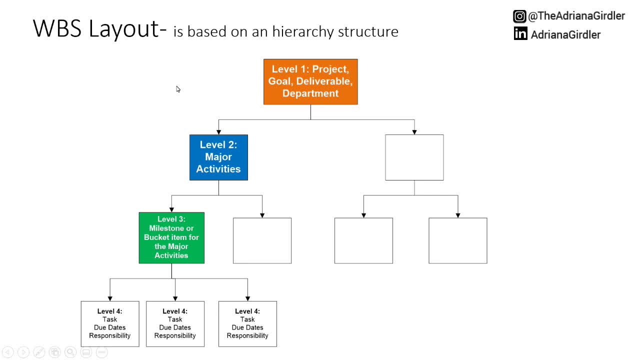 down in this manner. It's a super easy way to get a handle on the amount of work you have to do and to truly understand if you have your scope correct, your timing correct, etc. So really break things down. If you're in a WBS, there's a lot of work to do. So, again, if you're in a WBS, you have to. 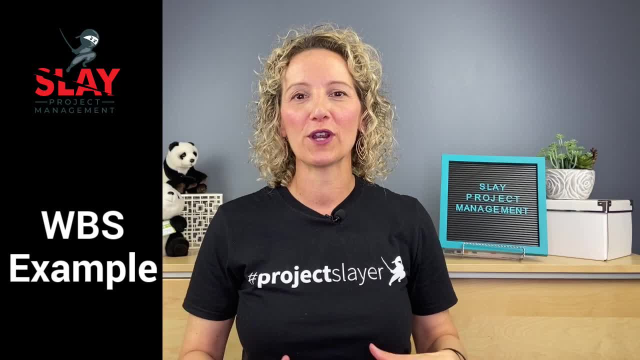 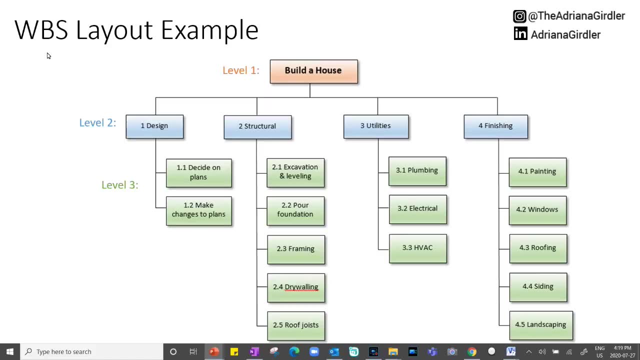 be very, very, very careful about this. So one of the things that you want to do is to build a layout in a WBS with level one, two, three and four Work breakdown structure example. So I have an example here for you on a construction project. Okay, so now let's actually take a look at an 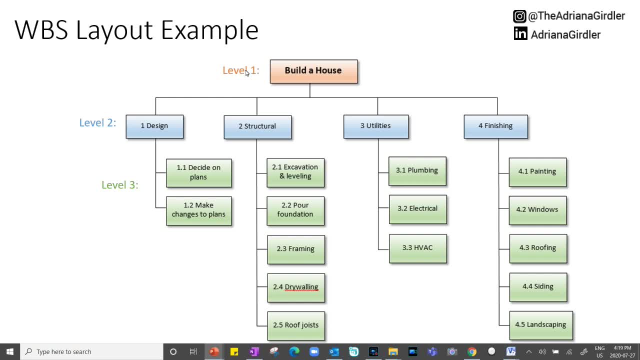 example, because when you see it, as you can see what I have in front of you right now, it really makes a lot of sense. So that level one: what is our deliverable? It's building a house. Now, you can only imagine how complex this can be. So what are our level twos? Well, with this project, 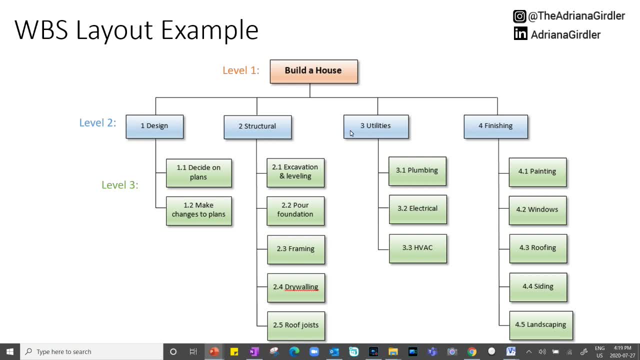 particular way it was broken up. it was in design, structural utilities, finishing, and now this is where the level three. there's even more you could break down within that level two. and so if you take a look, for example, of design, decide on your plans, make changes. let's take a look at some utilities, so you have your. 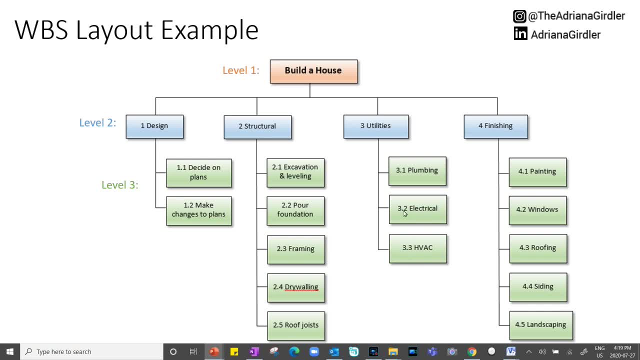 plumbing and your electrical and your HVAC. now one more level that is not shown here is your level four. so underneath plumbing you're gonna have tons of tasks. just to get all the plumbing one would be: take a look at your plan and get a list of all your plumbing materials, go to the store or put in the 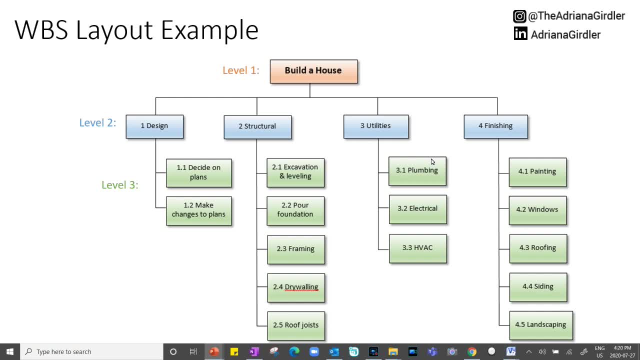 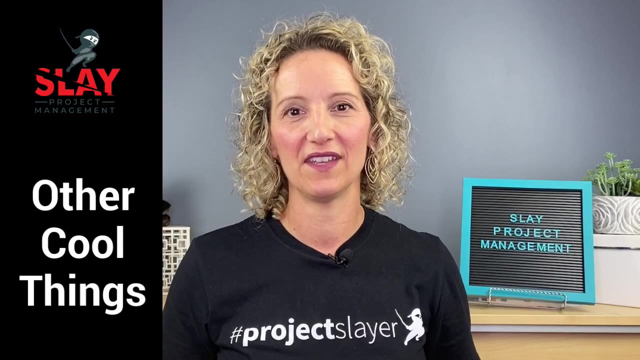 order for your plumbing materials. pick up the order from the plumbing materials schedule in your plumbers in order to put in the material. do you see what I mean? there's a lot that you can do here, but it just shows you how you can break things down, as I like to say, in manageable chunks. other cool things: 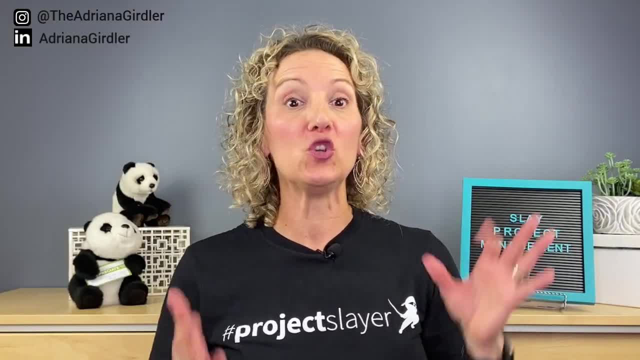 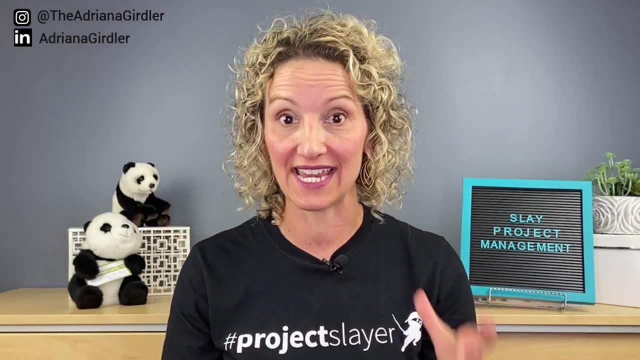 about a work breakdown structure. all right, the first thing that you need to know about a work breakdown structure is that the first thing is you can take this structure that you just created and translate it into an action plan. it is an amazing tool and technique to do this. 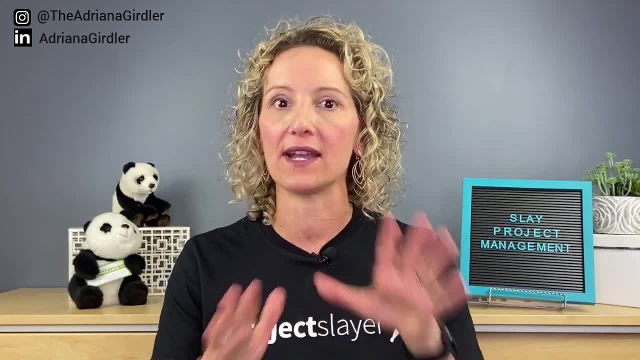 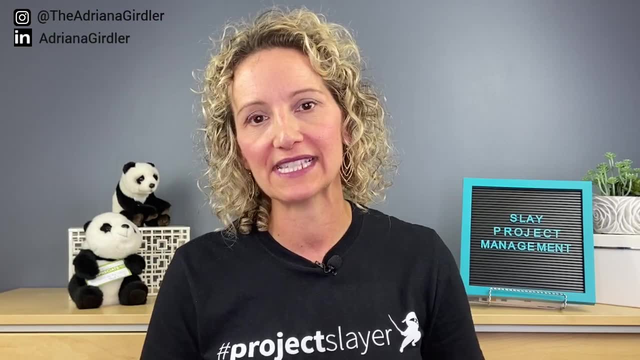 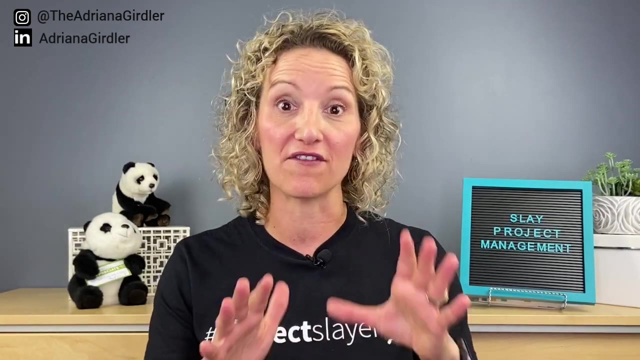 and actually pull it all your action items, so something that I highly recommend that you do. another cool thing about WBS is it actually can bring accountability to your team members, because this is something that you should be doing with them and, last but not least, use it as an activity creating. 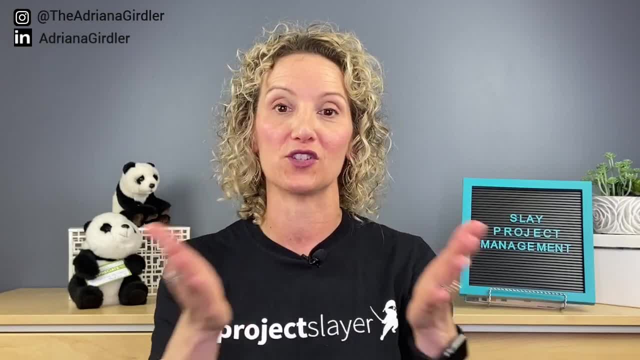 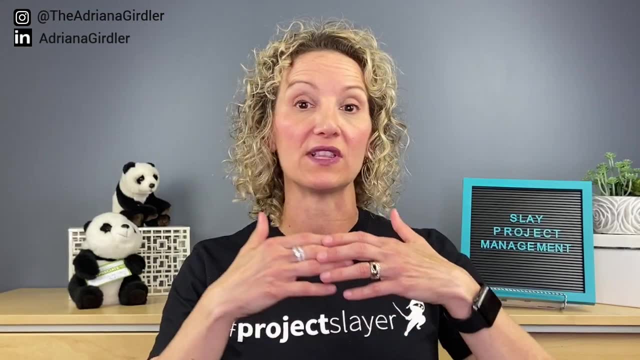 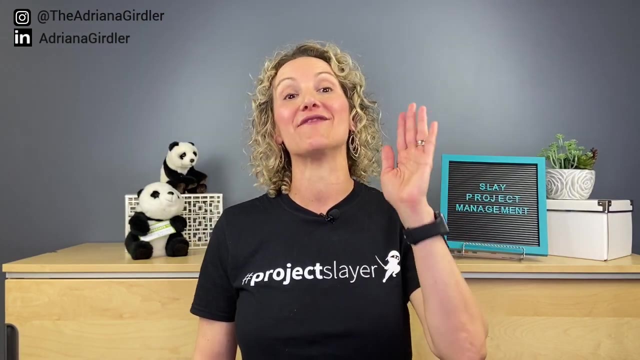 and finalizing your WBS, particularly if you create it into a project plan at your kickoff meeting. so cool this tool. it is so important to project management because you use it throughout the lifecycle of a project. now that you understand all about work breakdown structures, it is time to go even deeper. 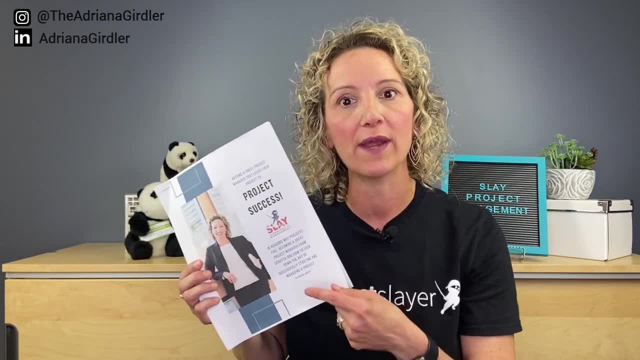 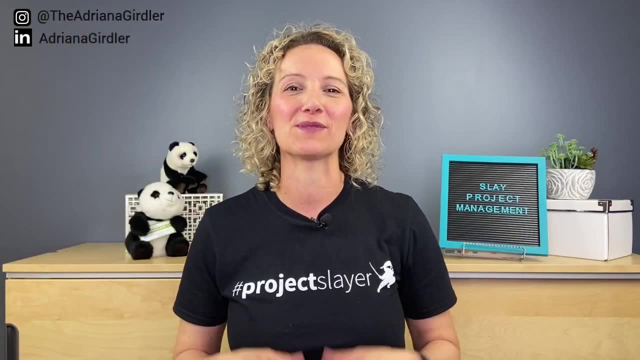 into your understanding of project management, and that is this why projects fail. you need to ensure that this does not happen, so go to the link below and grab this document. don't forget to subscribe and like this video. share with all the people that you know. tell me, are you? 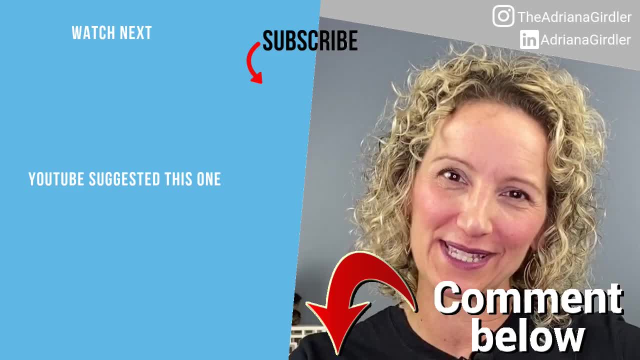 more confident now in creating a WBS. I'd love to hear from you. please put it in the comments below. until the next video, see ya.